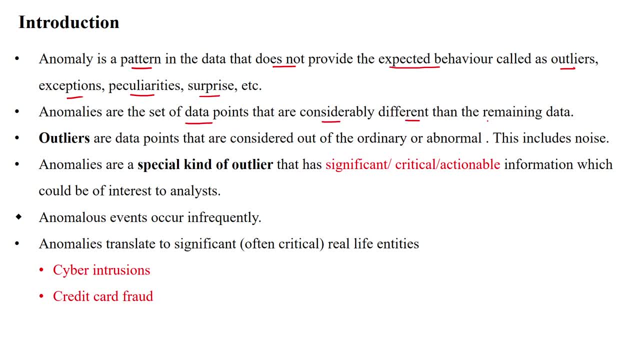 points that are considerably different than remaining data available in the data set. The pattern of the outliers and normal data points will be different Here. outliers are data points that are considered out of the ordinary or abnormal, So it includes the noise that means the abnormality is occurring due to the noise included in the given data point. 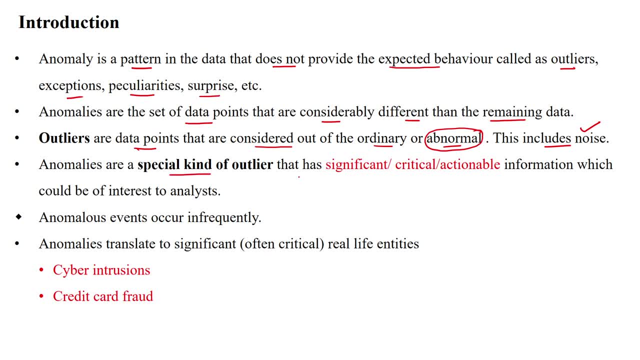 Anomalies are a special kind of outlier that has significant or critical or actionable information which could be of interest to the data analysts. Anomalous events are occurring infrequently. that means rarely, which is occurring. in the events, The anomalies are translating to significant. 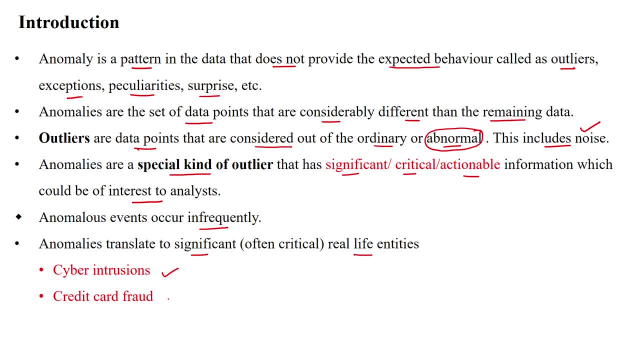 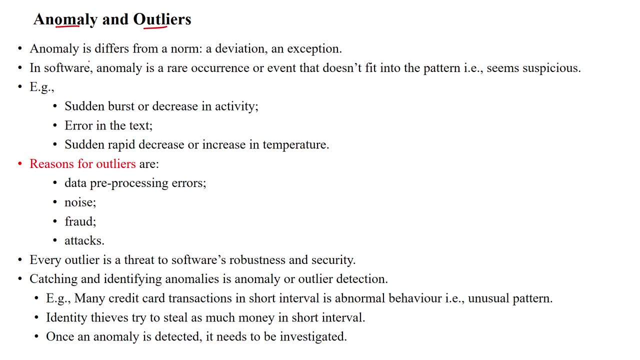 real-life entities, for example, cyber intrusions, credit card fraud and so on. Anomalies are different from normal activities. that means it will have slight deviation or exception. In software industry, anomaly is a rare occurrence or event that does not fit into the regular pattern that. 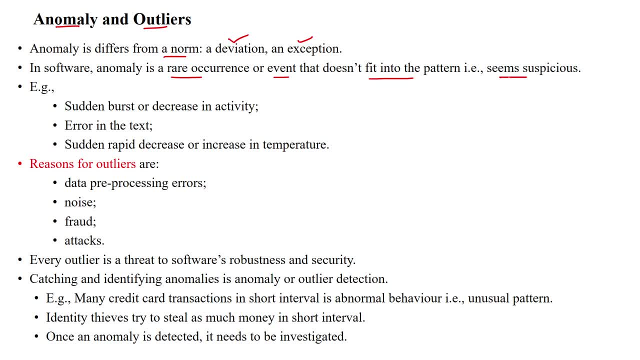 means, it seems, suspicious activity, suspicious event, For example sudden burst of a car or an accident. Here it is not a warning for outliers, But if the outfit movement is a very active activity and an error in the particular text, or sudden rapid decrease or increase. 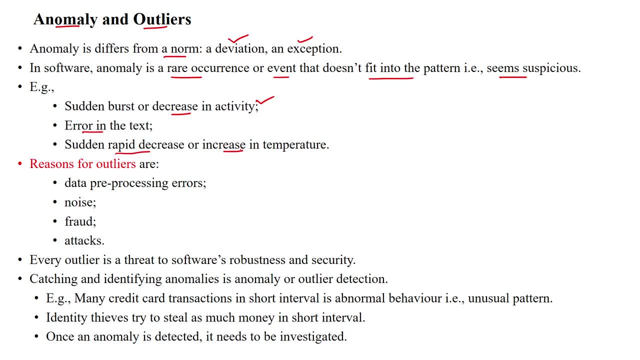 in the temperature of the CPU or any computer systems, then it is a very. these are the things that we need to take into consideration. In our case, when we are talking about outliers in a device, what we are talking about is the error in data preprocessing, just because of the error in the data or any mishandling. 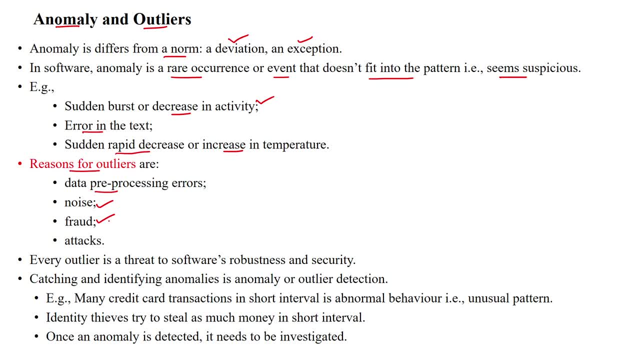 or fraud of any kind. We cannot say for certain types of outliers are outliers and we cannot even say for certain modifying the data, modifying the programs by use by opponents, and also there is the possibility of attacks. so these are the possibilities for making the outliers, or i mean occurring, the 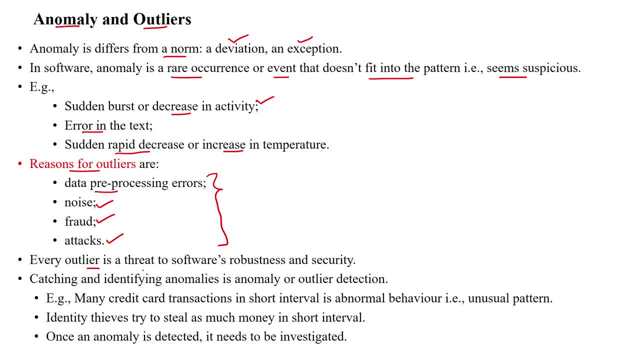 outliers in software industry. every outlier is a threat to software's robustness and security and catching and identifying this anomalies is called anomaly detection or outlier detection. for example, many credit card transaction within short interval is called abnormal behavior or it is called unusual pattern. that means if any person is having the credit card, the 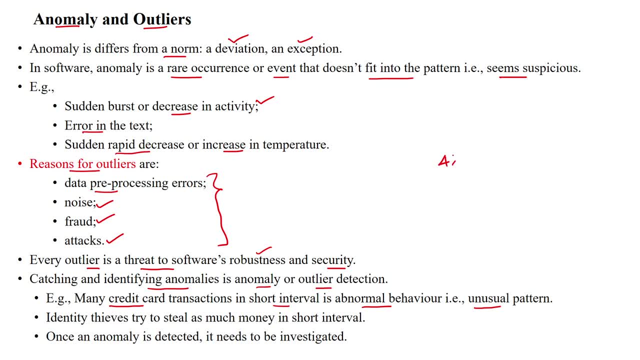 credit card limit is, for example, four lakhs, then he will use only fifty thousand or one lakh for in the single transaction or two transactions, but uh, uh, for each transaction there is the limit, for example, uh, fifty thousand. so if it is the for single transaction, uh, having the limit, uh, uh, fifty thousand, then the, if any up any. 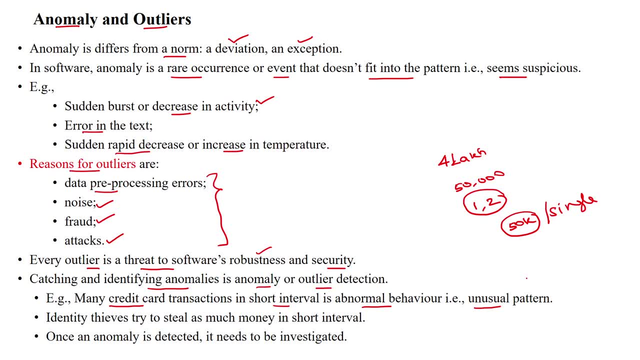 unauthorized person is uh- uh, i mean hacking your uh credit card, or he has hacked your pin number, then he will try to get all entire four lakhs of four lakhs amount within the short interval of time. so this is the limit for each transaction. for example, fifty thousand. 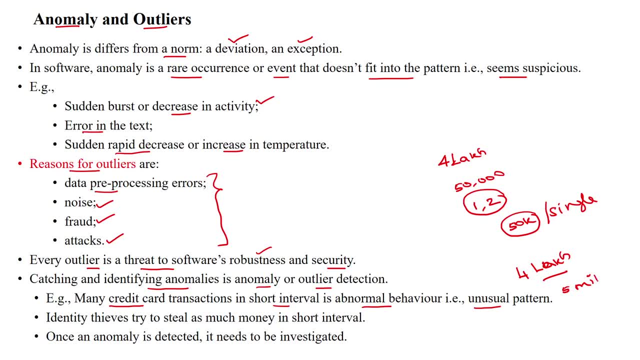 short interval time, within the five minutes or ten minutes. so this type of transactions are called uh, unusual pattern or abnormal behavior and identity uh of thieves, which are uh who are try to steal as much as money in the short interval, that is the uh given within the 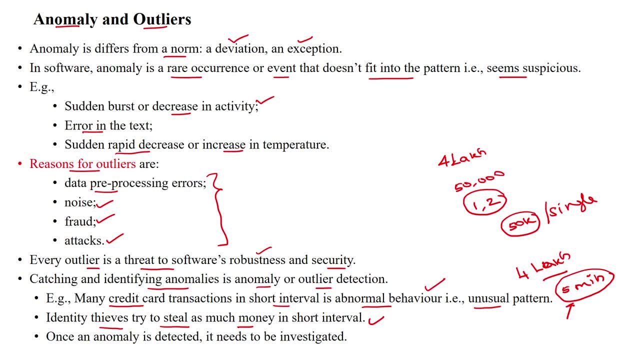 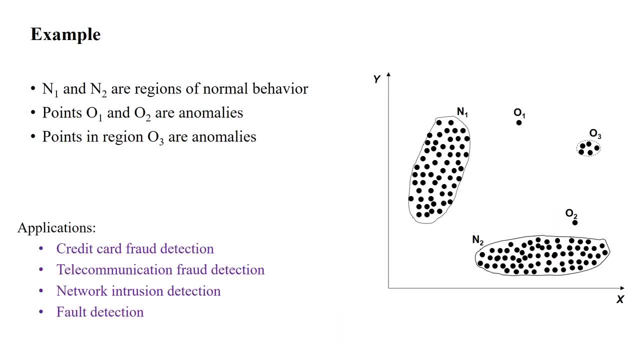 short interval, five minutes of time. so this kind of things are called uh outliers or anomaly behavior. for example, in given a data set which is having uh the clusters, i mean a different group of data here, different clusters. you may. you may assume these are all your uh clusters. so here, uh n1 and 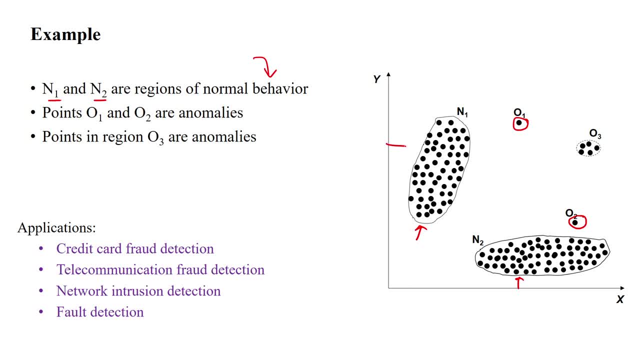 n2 are the region of normal behavior, because, uh, this, uh data are having dense clusters. that mean dense data data samples. but here this one is having only single data point and the other one is having, which is having five data points. this is having single data points, so these are all called